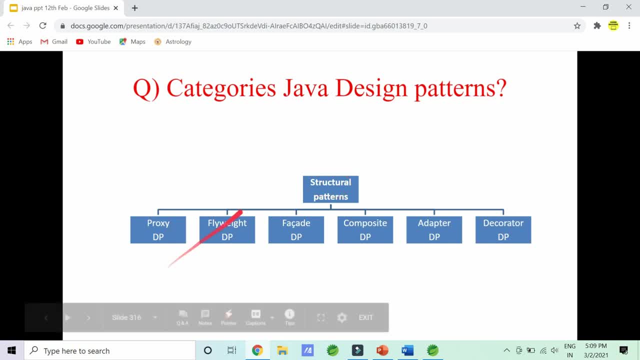 design pattern. You can categorize the structural design pattern into six parts. The first is proxy design pattern, Second is flyway design pattern, Third is facet design pattern, composite design pattern, adapter design pattern and decorator design pattern. So let's quickly. 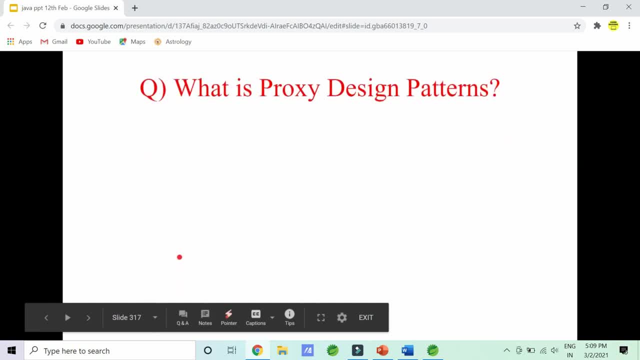 move ahead to the proxy design pattern first. The first question that may arise is: what is proxy design pattern? So proxy design pattern is nothing but a structural design pattern. I've covered this already. It will let you provide a substitute or placeholder for another object. This is going to be theoretical, but 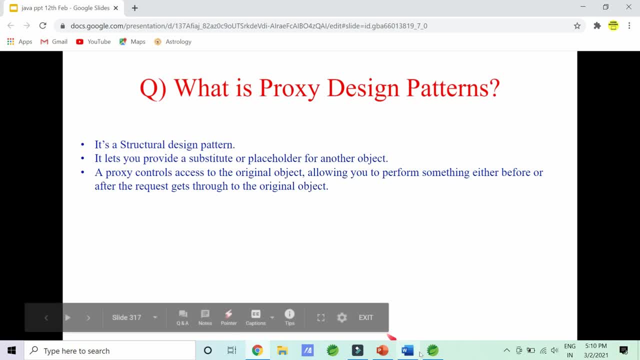 let me quickly move to the demo part so that it will help you understand better. But first understand that the proxy is nothing but a way to access, control, the access to the original object. So when you are into a college, when you were into college, when you were in college, when you were in college, when you were in college, 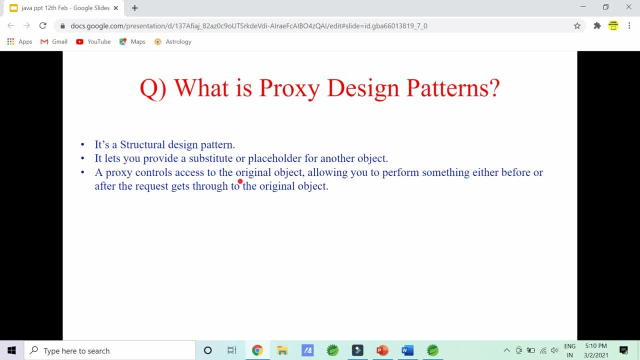 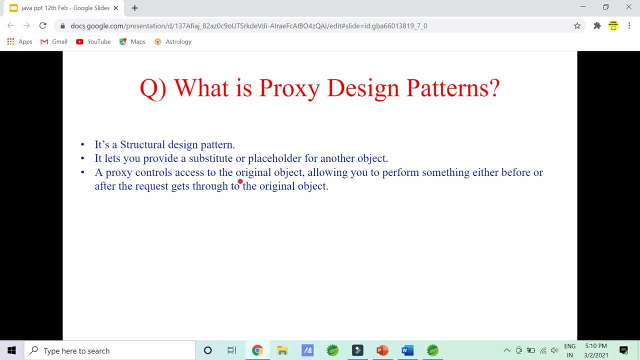 a proxy saying that I am the original person. First contact me, Then maybe the person whenever is available, it will put the attendance. So proxy is access control to the original object, allowing you to perform something before the request goes to the original object. 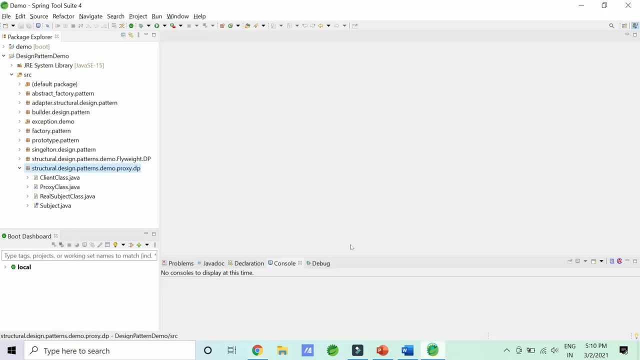 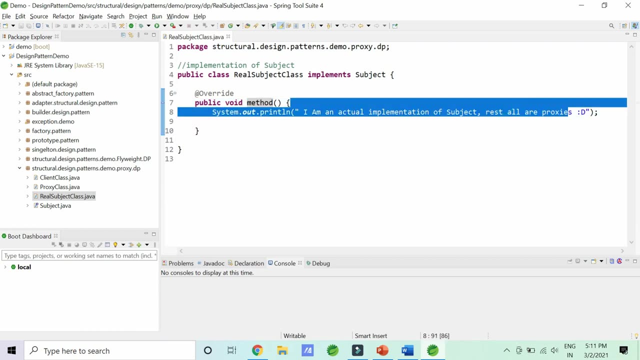 Let me quickly make you go through the demo first, so that it will be easier For you to understand. So this is my real object. Okay, It has a method. I am the actual implementation. rest all our proxies. The proxy class will say: hi, I am proxy. First, I will. 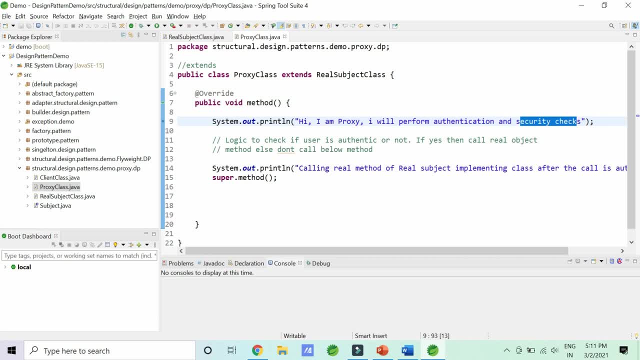 perform the authentication and security check. If you pass your authentications and security check, then only I'll call my parent or the one I'm extending the parent class method. If it does not pass, then I'm not going to allow you to put anything into this method. 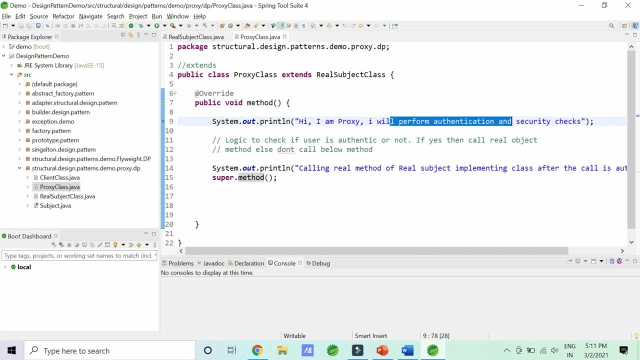 or call anything into this method, First pass my authentication and security. So basically, in the real implementation, you will always put this in if and else condition: If your authentication security check is passed, then call this method. else throw in error message that you are not authorized or your security check does not provide any authentication. 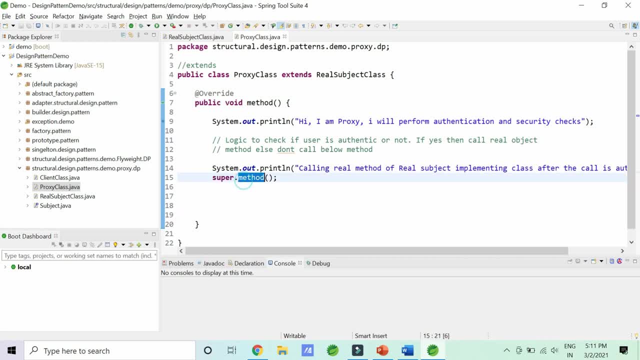 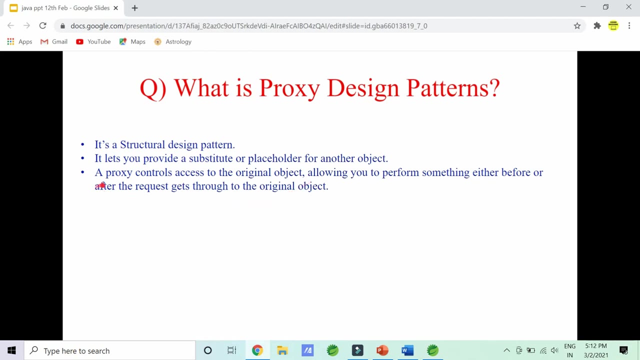 so that you will be able to go to that particular class and call its method. So this is a work of proxy. Proxy prevents the real method call or the real objects method call and it first check: Are you authentic? If yes, then only go, else, get out So proxy. 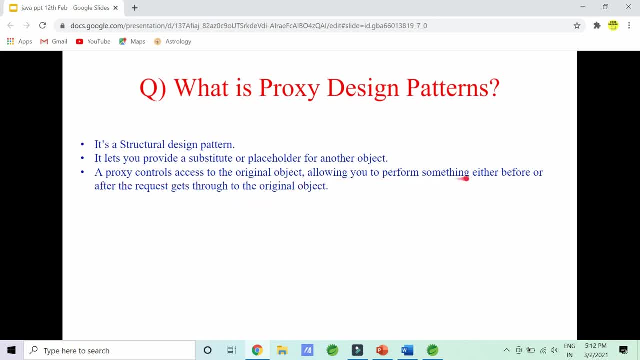 controls the access to the original object, allowing you to perform something either before or after the request gets through the original object. Now, first let me tell you the architecture of proxy design pattern. So the proxy design pattern architecture says there is a client. 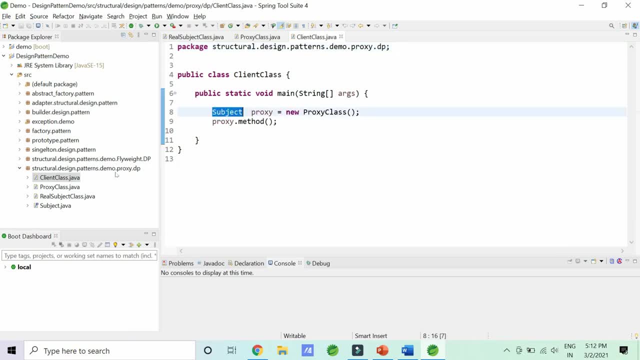 So let me tell you where is a client. This is my client. So what client does is. first let me tell you what a subject. subject is nothing but an internal object. So let me tell you what a client is. So what client does is. first let me tell you what a subject. 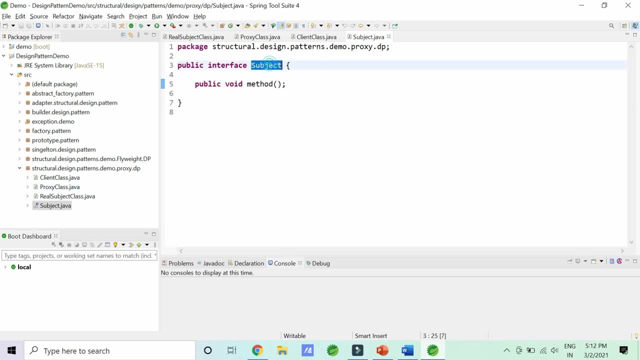 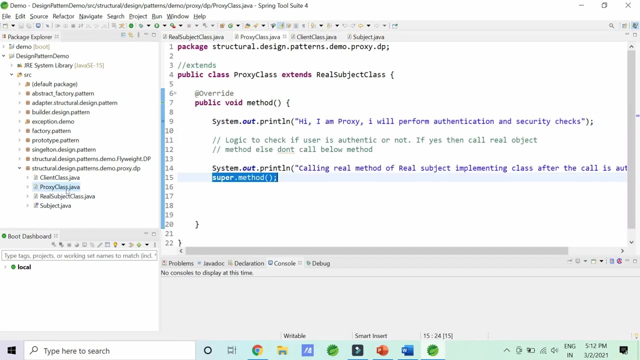 interface having one method. now this interface method, subject will be actually implemented by the real object, real object class. now real object is having a method which is having the actual implementation of subject. rest all our proxies, then I will have a proxy class which extends this real class. it. 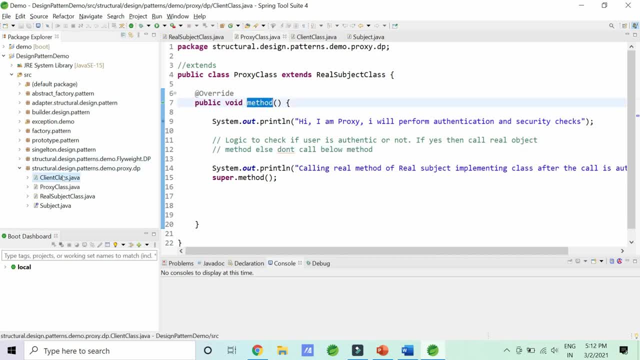 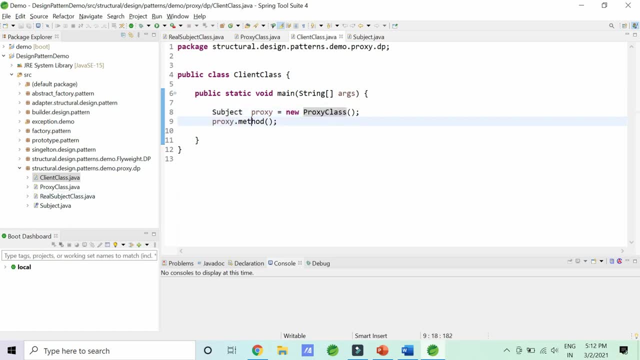 will, whenever you try to call this method, you will in the client class create an instance of a proxy class and not the real class, and then you call a proxies method, dot method. so if I try into this, it's a subject method, so you cannot directly get into the proxy object method. so this is one level. 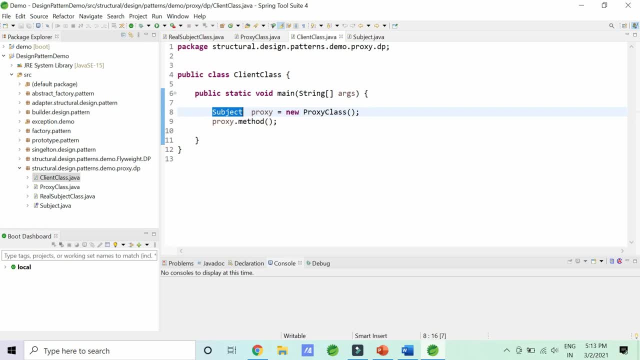 security. we are creating an instance of a subject which is an interface, so parent reference, class or memory. basically new provides you the memory. so the reference is of interface. memory is given to the class, but not the real class but to the proxy class. so whenever in the runtime, whenever this method goes, it goes into the proxy class method. this 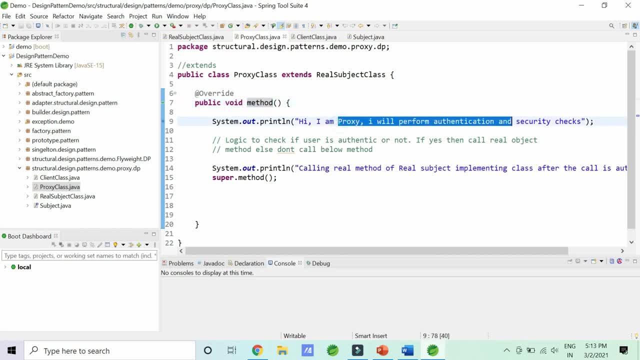 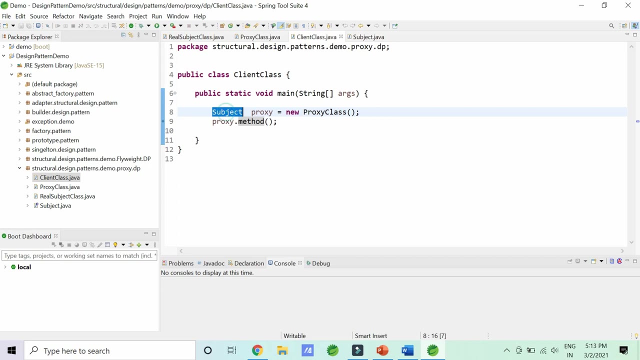 method, which is a overridden method. it checks whether everything is safe or not, and then you call it to the real objects class method. this method- okay so, if this is clear. so client class is doing nothing but creating the reference of an interface which is implemented by real subject. 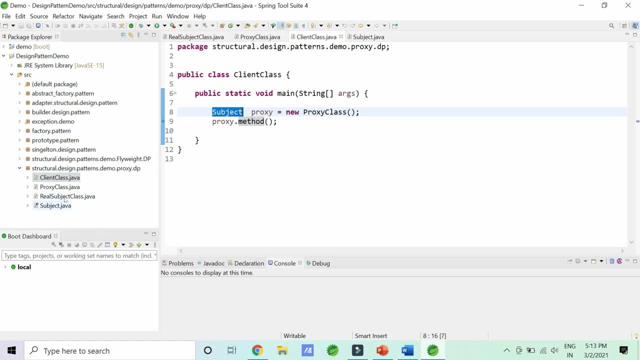 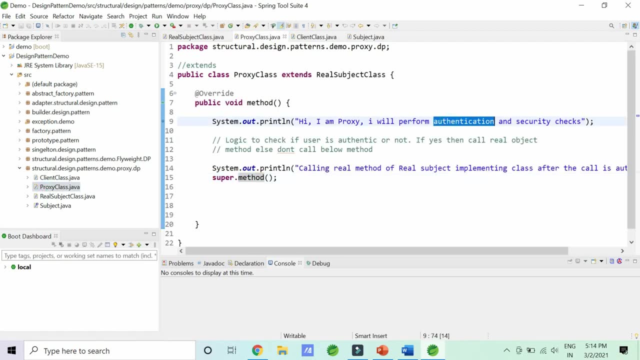 class, which is extended by proxy class. and why so much of complications? why not directly? because you want to first check whether you are authentic or not. if yes, then only you are able to access the real class. else you are not eligible to access any of the method of the, the parent class, the parent class or the. 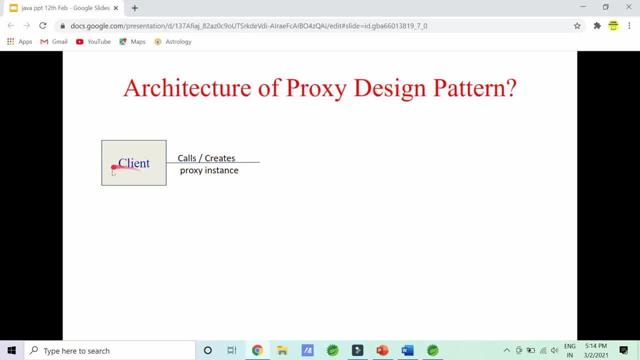 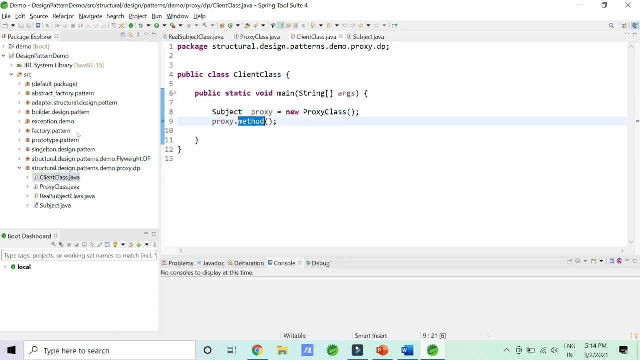 real class. so how does the architecture goes? architecture goes that client should always create a proxy instance, not the real object instance. so the proxy object is once and then proxy object. so here your proxy object is created. proxy object method is called. in the proxy method it will check whether you are authentic or not. so method calls of a real. 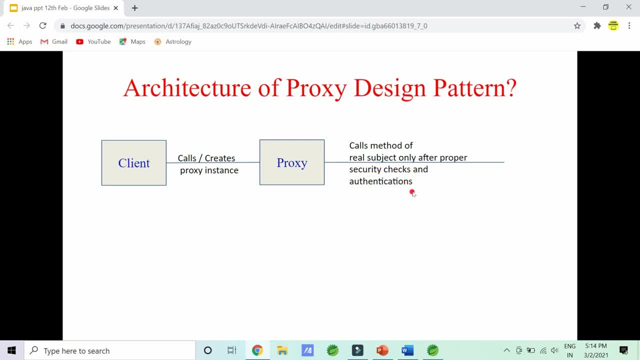 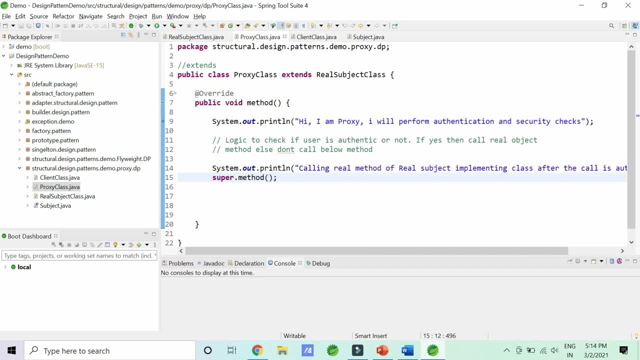 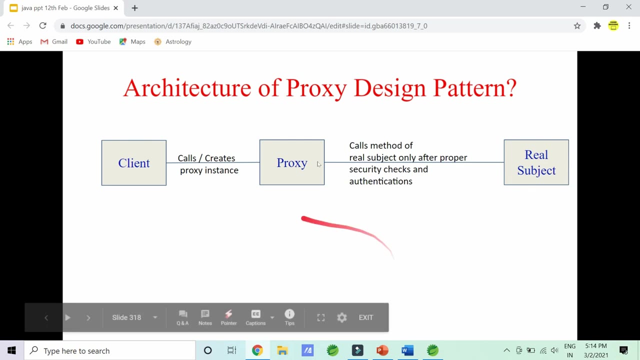 subject only after proper security check and authentication. if you pass the authentication, if you are actually passing this authentication, you can actually call the real method. what does super? super is nothing but the real object. so once you pass it, the next real subject is called. if not, you are thrown back saying you are not authorized. so if this much is clear, let me quickly make you. 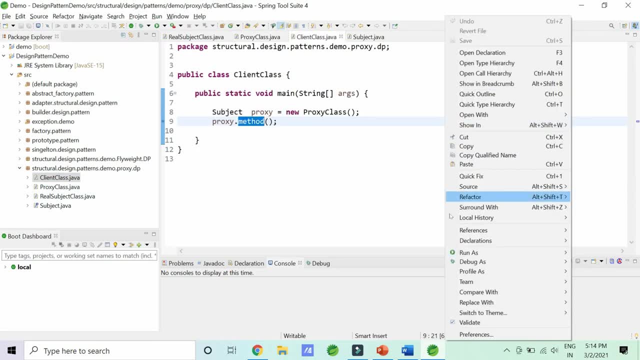 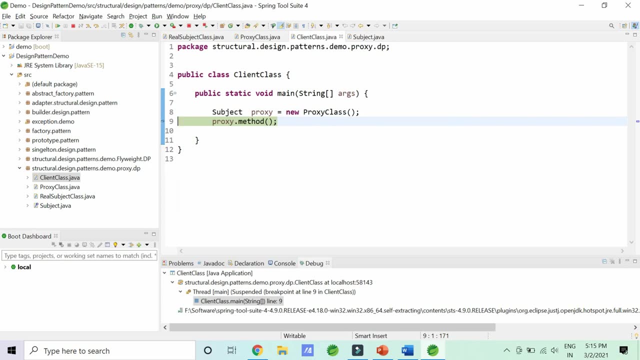 go through this particular code base by debugging it so that it is clear to you. okay, so whenever this proxy method is called, let me go into this and put uh implementation here. uh, i go into proxy class and debug is already here. so if i do, f6. 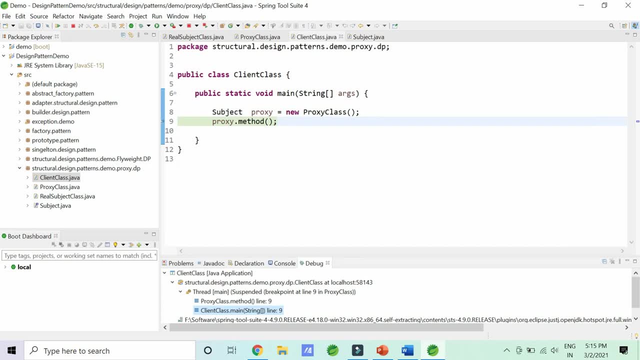 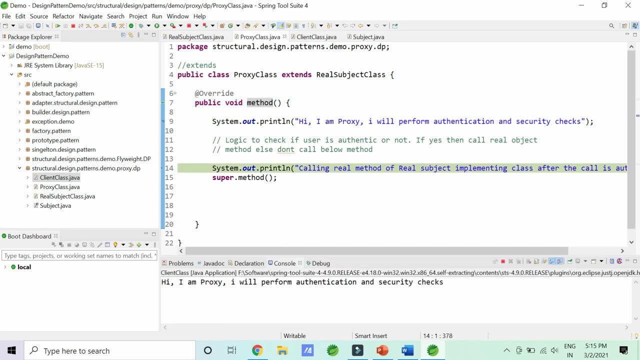 then okay. so if you say client, I was here, the proxymain method is called and then it goes into the proxy class method. it says: I am proxy, I will perform authentication and security check. now I am assuming that, yes, it is. it actually succeeded the authentication and the security check and now calling the real method of 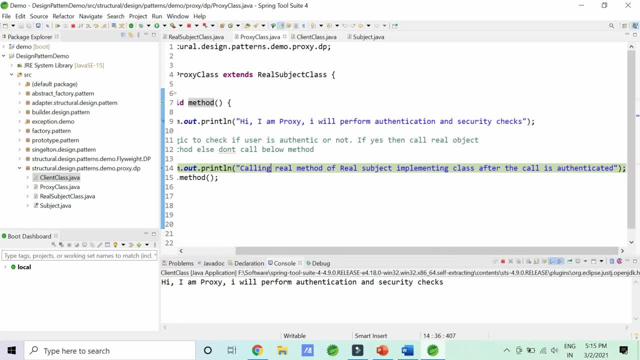 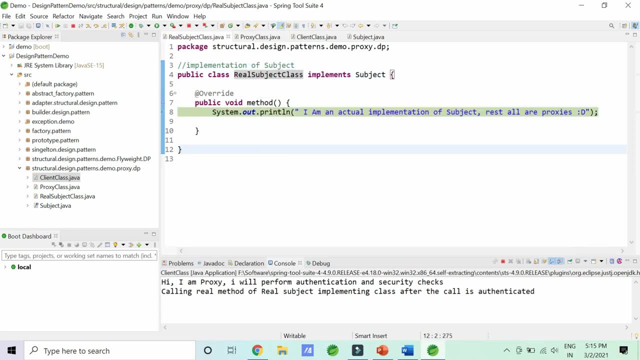 the real subject implementing class after the call is authenticated. and now my supermethod is called, so let me get into it. so now my real subjects. I am the actual implementation of subject rest. all are proxies. so since I was authenticated, I was able to access the method of the real 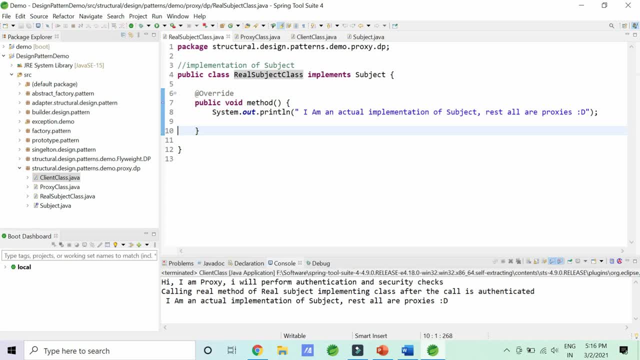 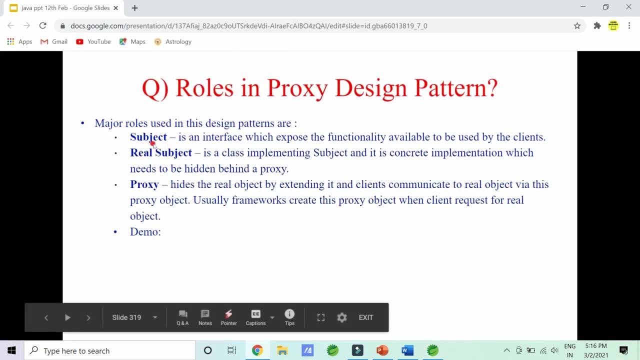 subject class. so this is how the real authentication goes, and that's all. if you are a proxy, you will perform authentication, then you will call a real method and this is the actual implementation. rest: all are the proxies through which you are getting called. so major roles in the proxy design pattern. 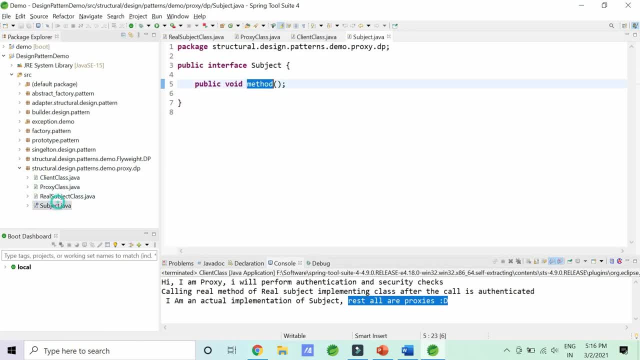 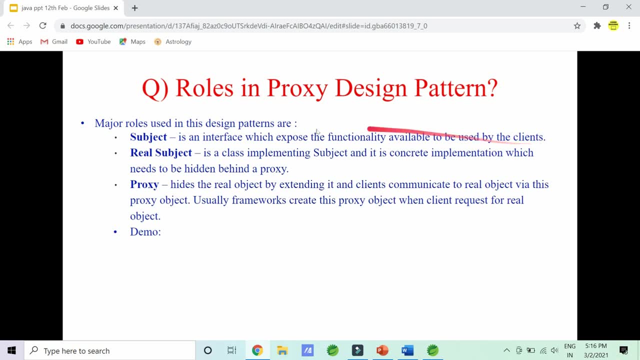 is called. so this is the actual implementation. rest, all are the proxies through which you are subject. so here let's go. what is a subject? subject is an interface with one method. the subject is an interface which exposes the functionality available to be used by the clients. so client wants to use a method functionality, what does it yours? so what is the? 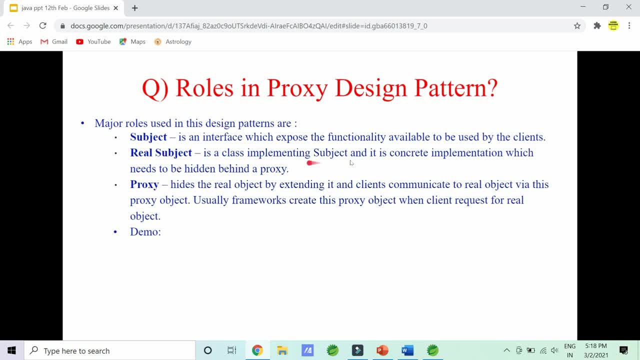 real subject. real subject is nothing but the class implementing the subject. so does it implement the subject? yes, it implements the subject, and it is a concrete implementation which needs to be hidden behind the proxy. so Proxy is the one who hides this. So how does it hide it? 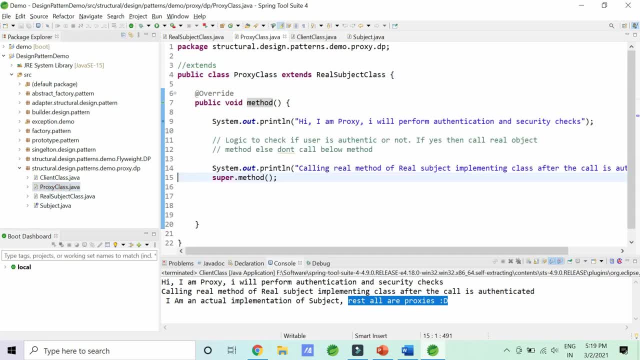 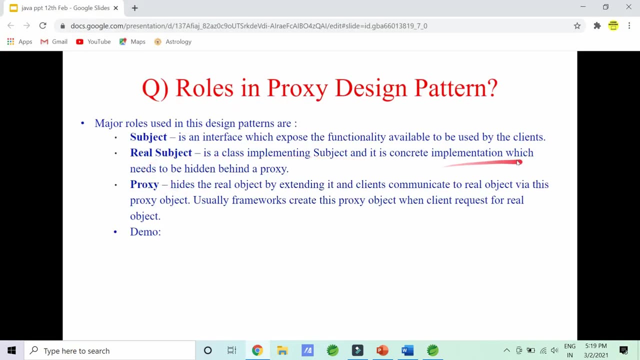 It actually extends this subject. What is a proxy class? It actually extends the real subject class and it overwrites it and hence it hides it for a time being. And it says: first perform authentication, then only go into the method. So real subject is having the real implementation or the concrete implementation, and it is hidden by a proxy. 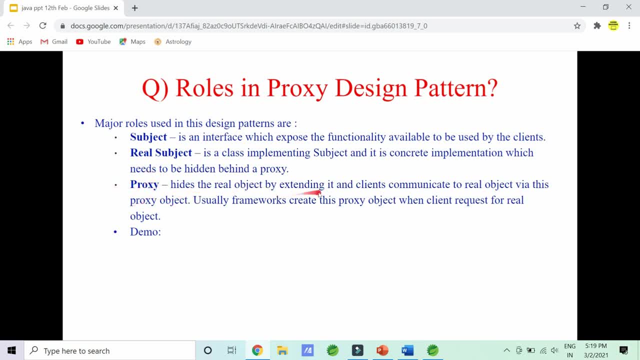 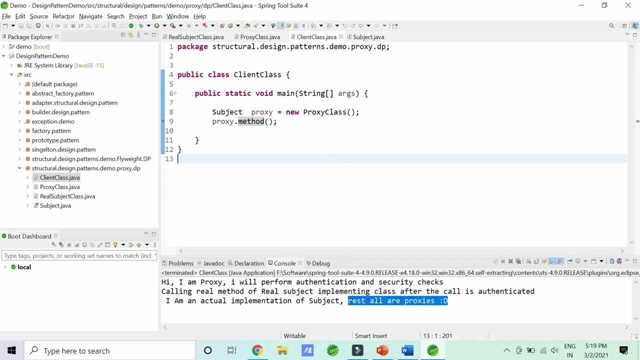 Now what is proxy? Proxy hides the real object by extending it. So does it extend? Yes, it extends the real class and the client communicates to the real object via this proxy object. So in the client you always create a proxy class and you call the proxy class only. proxy class method only. 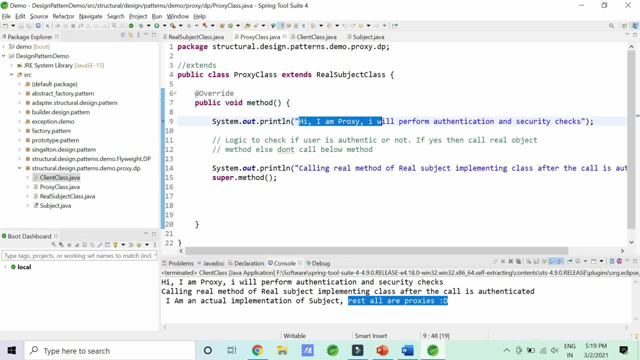 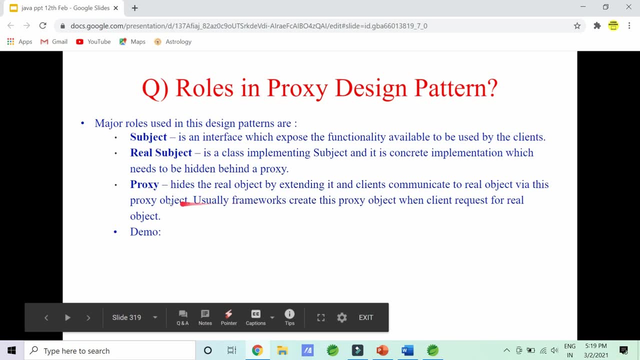 So in the proxy class method it says hide, perform authentication, then go into this particular real object. So proxy is used to hide the real object And the client. So the client creates an object of proxy class and usually framework creates this proxy object when clients request for a real object. 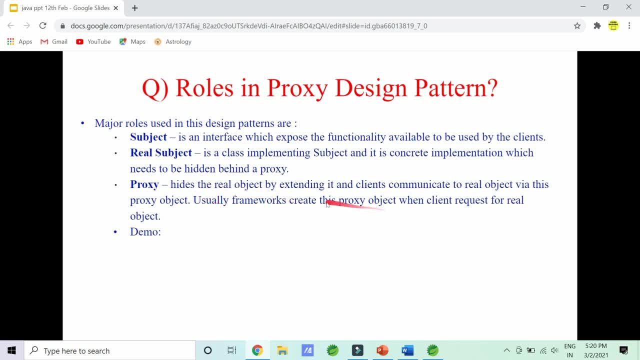 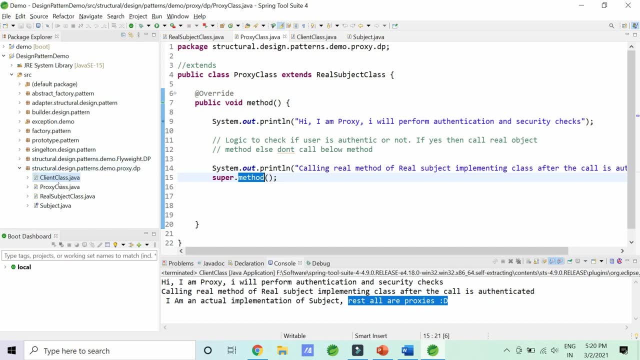 So this is the work of framework, that the proxy object should be created whenever client tries to request for the real object. So it is a work of framework to do this particular thing, To create always a proxy class, call the proxy method. Proxies should check the authentication. 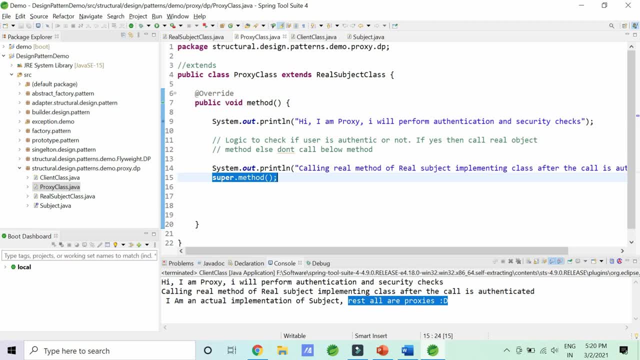 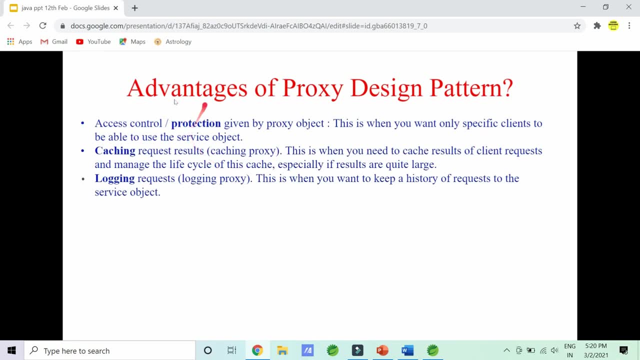 If yes, then call the real method, Else don't call the real method. So that was all about The implementation roles in the proxy design patterns. If that much is clear, let me quickly go ahead to the advantages of proxy design patterns. 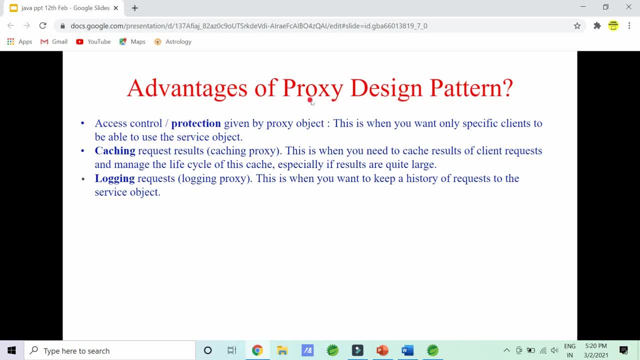 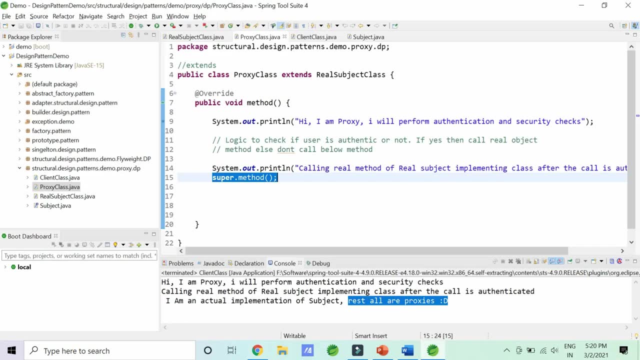 So this is a very important interview question. They will ask you: why did you use proxy design patterns? So the advantage is that you can provide the access control. So if you can see, here I have provided an access control. If authenticated, then only call the real method. 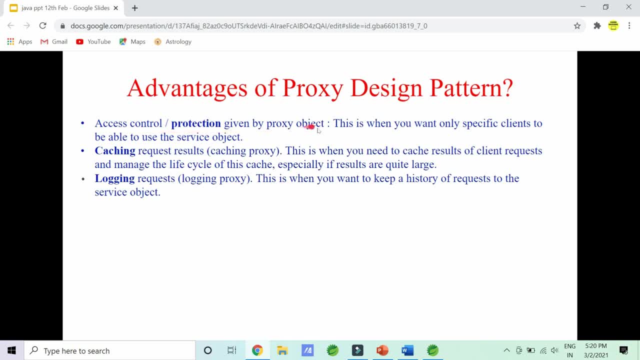 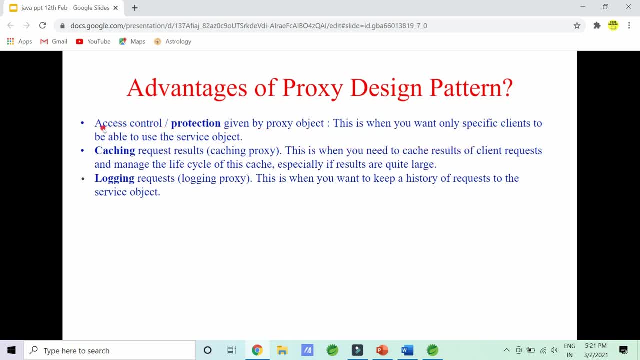 A specific client means the one who is having the access or who is authorized. Only those should be able to access your service. object: What is the second advantage? Caching is the second advantage, which is also called a caching proxy. This is when you need to cache the result of client request and manage the lifecycle of cache. 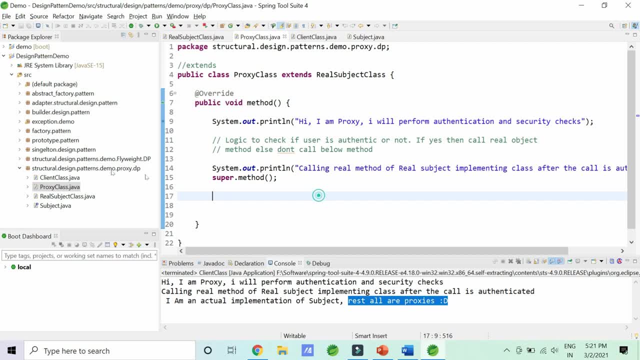 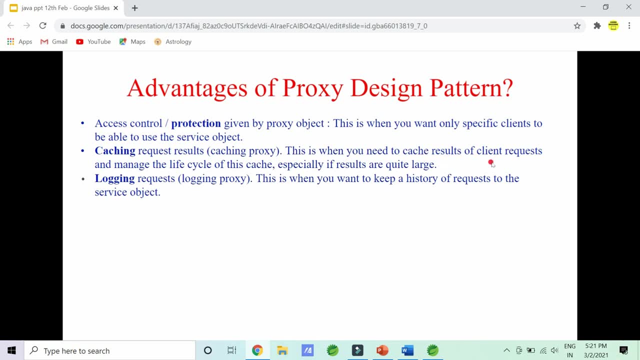 especially when the results are quite large, So you can actually cache your object. the responses in the proxy part. So this is: when you do your cache, You can, When particular response is quite large, you can always cache that particular result And the proxy will be able to give you, rather than actually calling the real object. 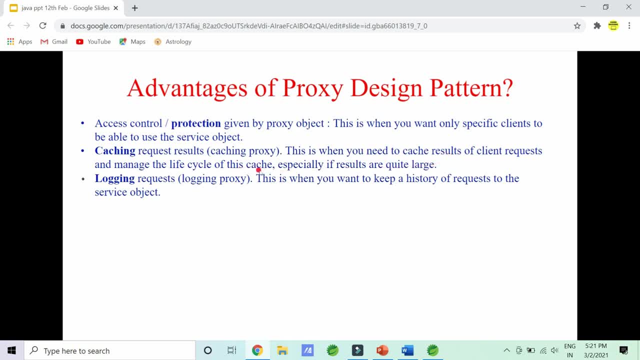 So that your memory and performance in time, everything is like saved. Logging request, So logging proxy. This is when you want to keep a history of request to the serving object. So this is very simple If you want to log. So what happens whenever a call to real method is gone? 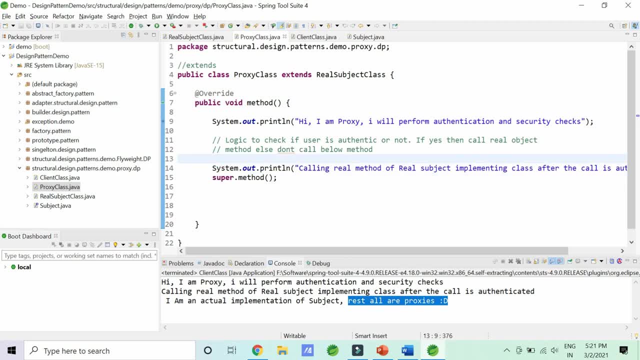 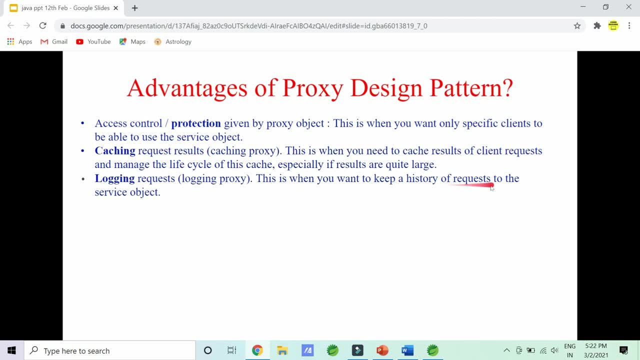 Here you can put a logger. So whenever a real A method is called, always a logging is done first and then a method is called. Hence you can always keep a track of how many requests and from whom is that particular object being accessed. 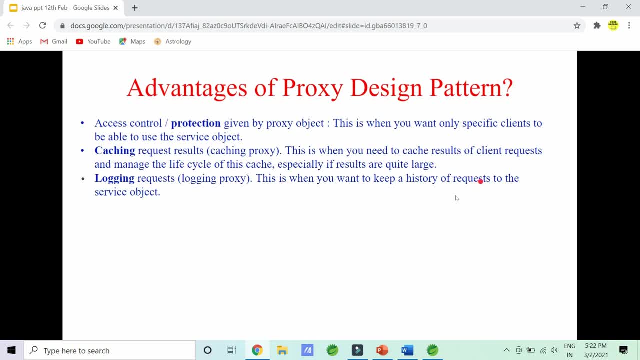 So that you can see if it is not being accessed by an unauthorized person through the logging purpose. So this was the logging proxy for you. So I hope this much is clear. If you have any problem in this particular proxy design pattern, please let me know in the comment section. 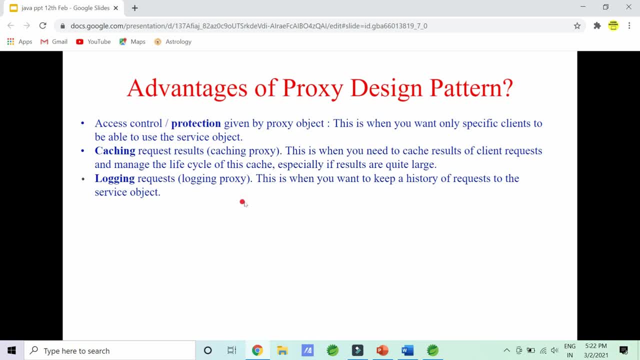 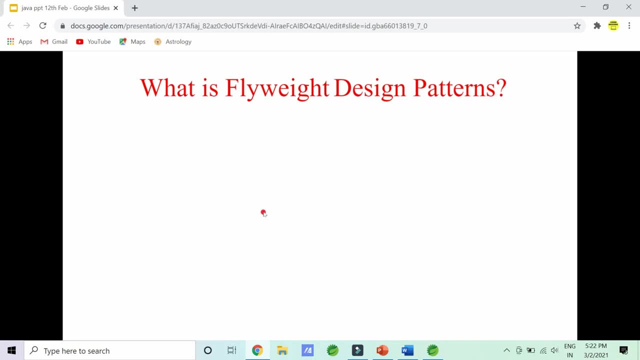 Because I expect, after learning all those five difficult ones, proxy will be a bit. I have tried to make it a bit easy for you. So if that much is clear, please let me move ahead to flyway design pattern. So I have already told you we have the six design patterns. 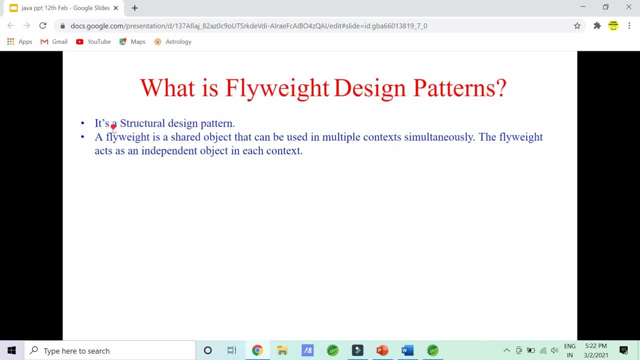 The second design pattern was flyway design pattern. So flyway design pattern is again a structural design pattern. A flyway is nothing but a shared object that can be used in multiple contexts simultaneously, So the flyway acts as an independent object in each context. 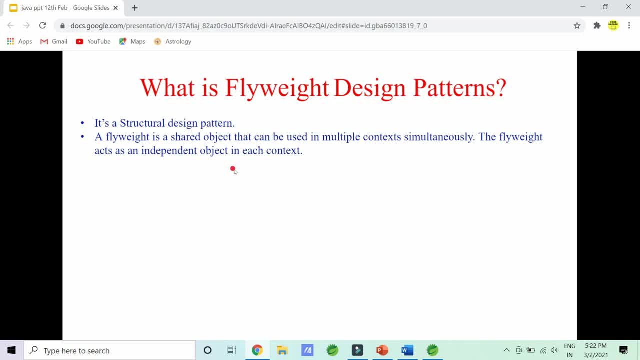 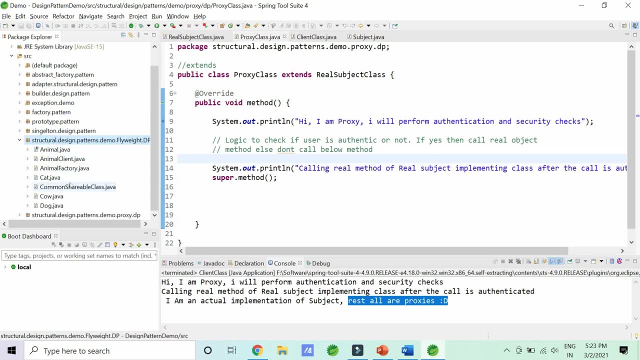 Gone everything. Didn't you understand anything? So let me give you a demonstration first. So because theoretically I understand, it's very difficult to understand the theory at once, So let me give you a common shareable class. This is a common shareable class. 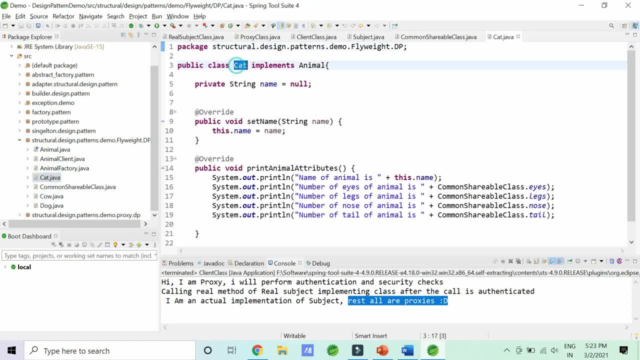 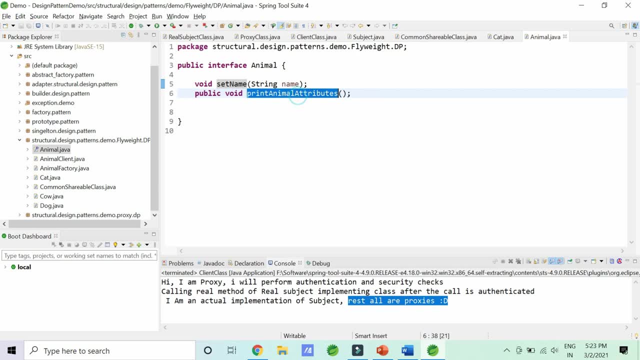 Let me give you an example of animal. So suppose a cat is an animal. So animal is nothing but an interface. It has two undefined abstract methods: set name and print animal attribute. Now I know that my cat, cow, dog, all of these animals are going to have. 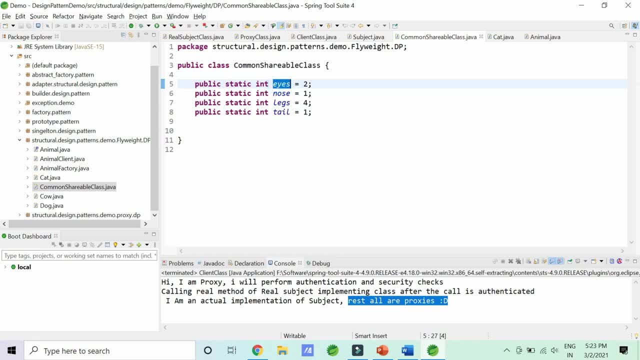 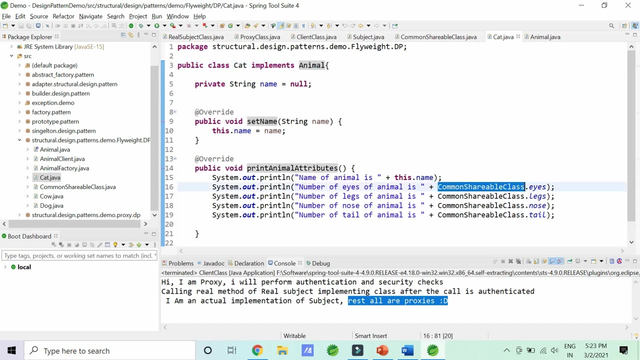 some shareable things, That is, they all will have always two eyes, always will have one nose, always will have four legs and always will have one tail. Exceptions are not included. Please do not include it here also. So cat actually implements the animal and then it has a common shareable property of eyes, legs, nose and tail. 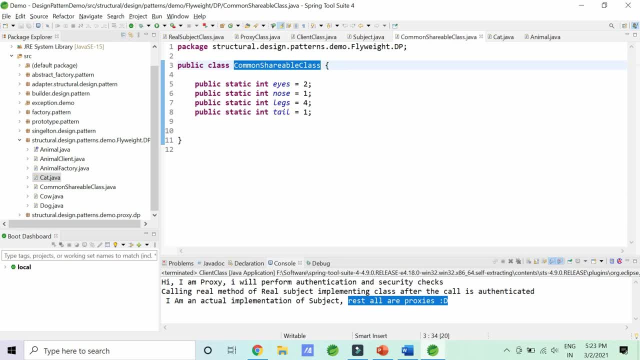 So I've maintained a particular class which is having the static variables And hence, once this class is loaded, all these variables will be shared. It will get memory as soon as class is loaded. So this is a Flyway Design Pattern. How is it a Flyway Design Pattern? 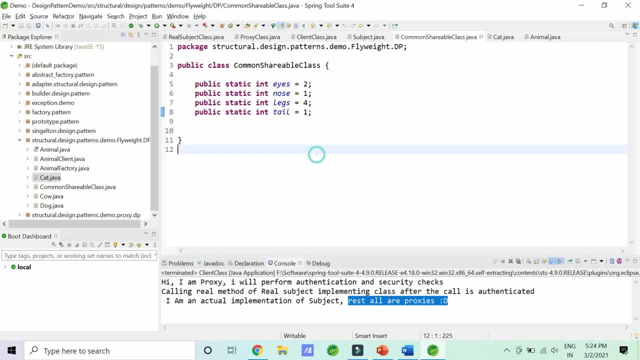 So Flyway Design Pattern is a shared object. What is my shared object? This is common shareable class Object is a shared object that can be used in multiple contexts simultaneously. Can't I use this common shareable eyes, nose, legs, tail in cat, cow, dog everywhere? 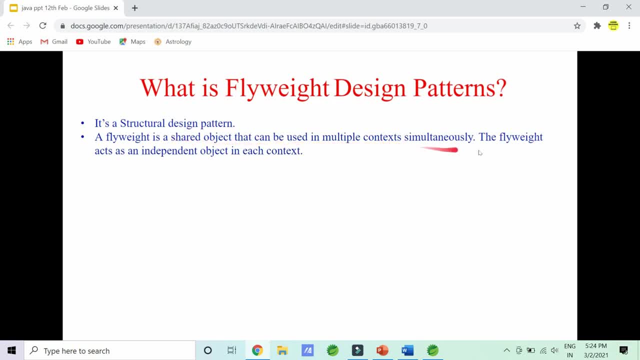 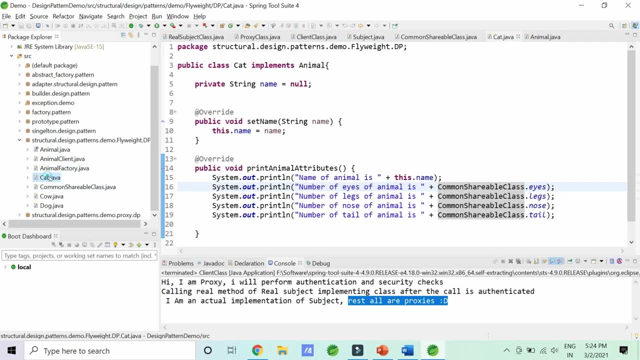 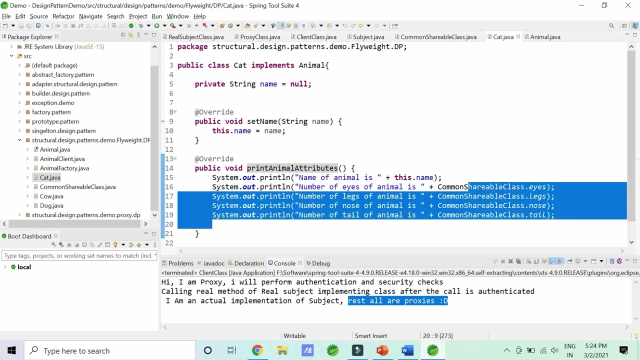 Yes, I can. Hence. it is a shared object used in multiple contexts and the Flyway Design Pattern X is a dependent object in each context, Every, every particular single thing. when I try to print the cat's attribute, it will have its own name and eyes, legs and nose as a shareable object. 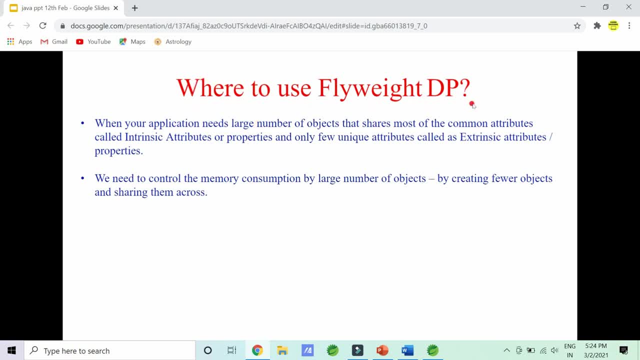 So if this much is clear, let me tell you where to use the Flyway Design Pattern. You can also say it as advantages of Flyway Design Pattern. So where do you need? See, you will have a particular program in your, in your hand. 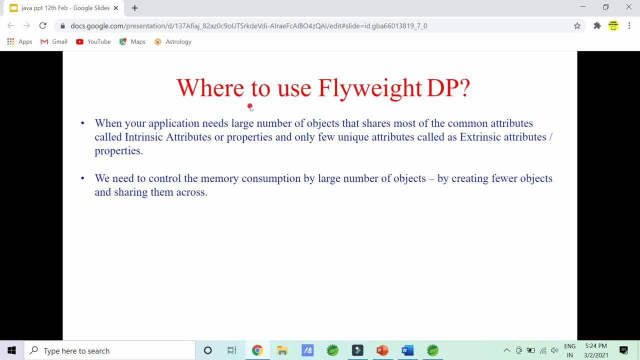 But to understand the issue and implementing a particular design pattern is what I'm trying to teach you here. So if you have an application which needs a large number of objects that shares most of the common attributes, then you can use the Flyway Design Pattern. 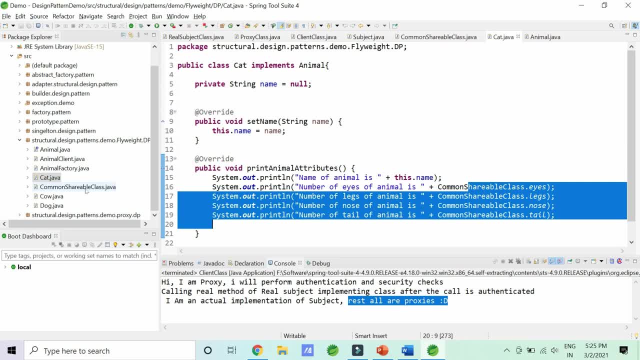 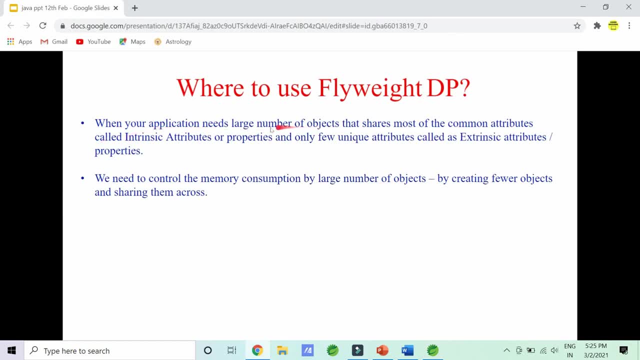 See, for example, if you have a very large zoo, I'll have multiple animals there. If your application is zoo management, you will have multiple animals there. Then, if there is a large number of objects, they share a common attribute. Say, for example, common attributes were eyes, legs, nose and tail. 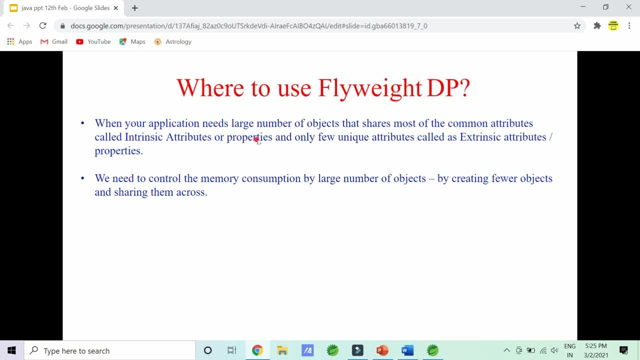 Then these are called intrinsic attributes or the properties. Please remember these two terms. These are very important from the interview perspective: Intrinsic attributes or properties, and extrinsic attributes, So which are common are called as intrinsic and which are unique are called as extrinsic. 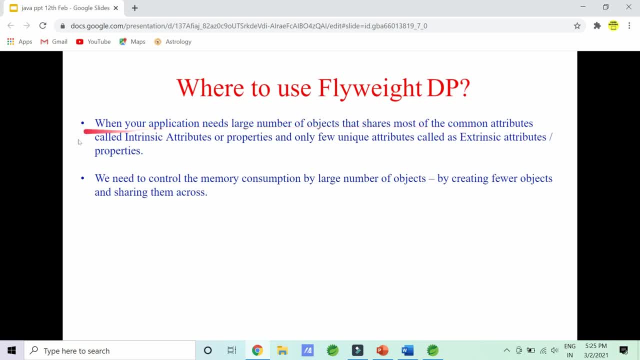 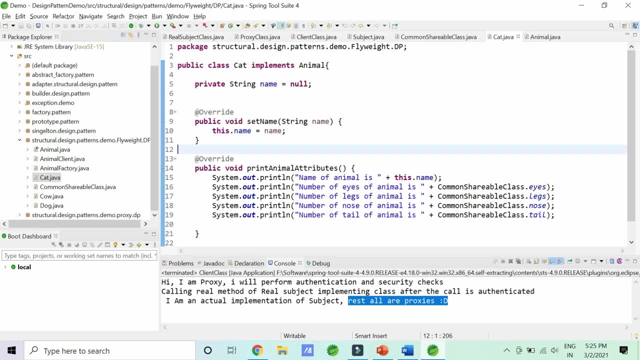 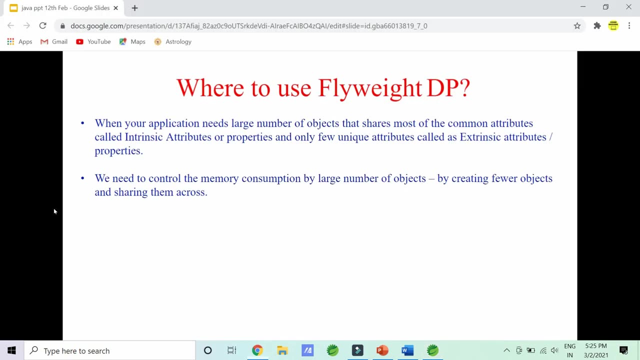 Currently, I've made it very simple for you. I have made only four common intrinsic attributes, which is eyes, legs, nose and tail, and only one unique attribute, that is name. So I'm going to identify the whole cat object with just a name, cow object and dog object with just name. 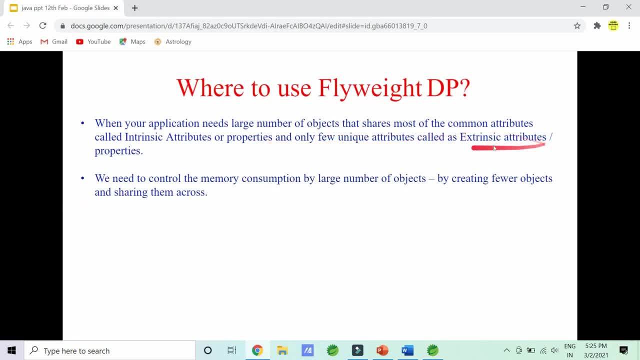 So for the making it easier for you, I have just one extrinsic and four intrinsic attributes. Now, when to use it? When you want to control the memory consumption by a large number of objects, by creating fewer objects and sharing them. So I'll tell you in a simpler way. 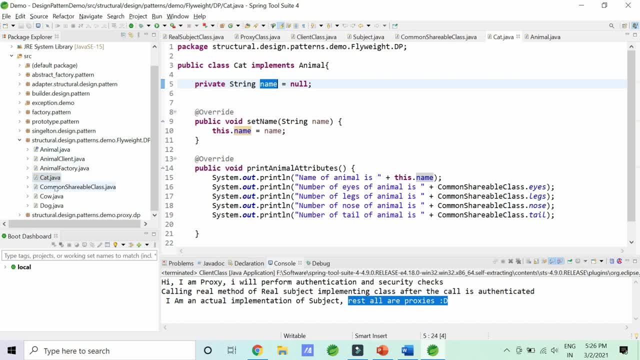 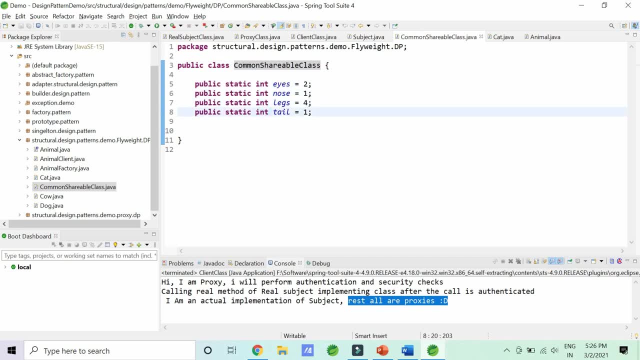 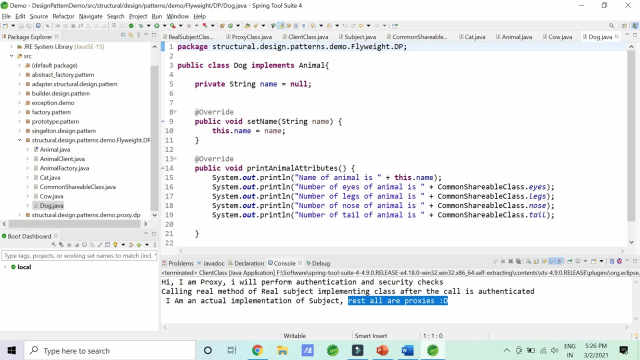 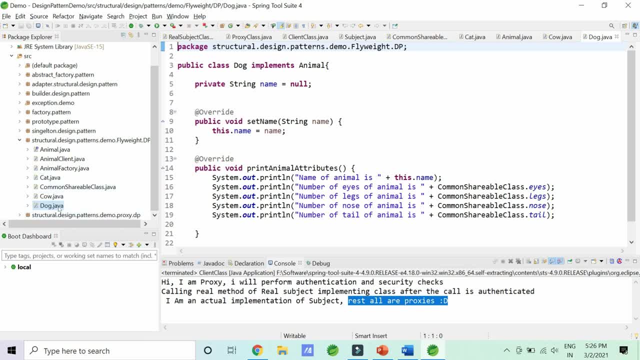 of only 16 by. the same thing is repeated for all the classes. So to prevent the memory utilization and consumption. and suppose I have 100 animals, all of them will have these 16 to 16 to 16.. How many? It's a large number. 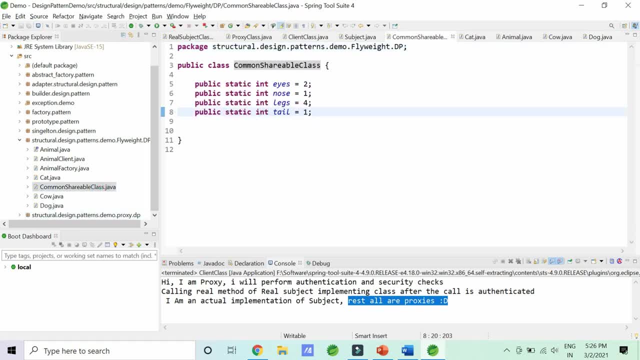 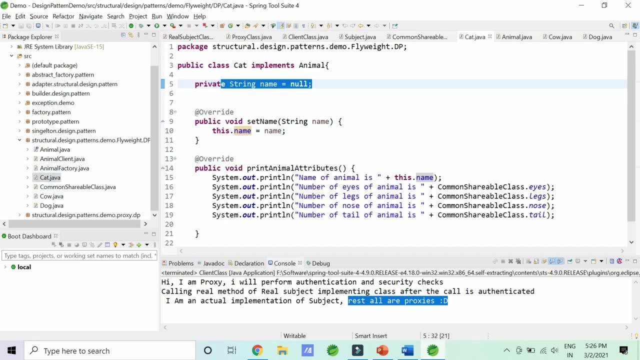 Why to do that? So do one thing: Create a shareable class, create at one place in a static manner, And then use it in this way. It's only string name will have the memory. Say, suppose I'm X, number of bytes, and then rest 16 is like saved. 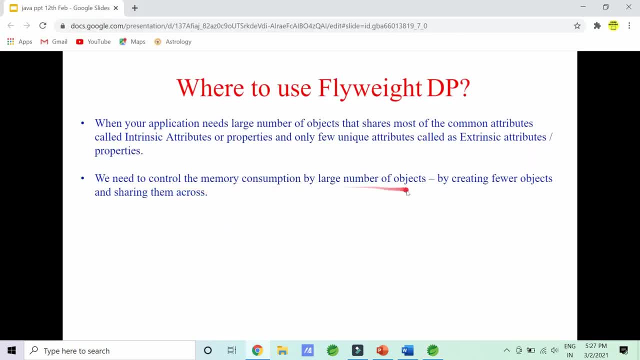 So can you see, there's a control of memory consumption. when you have a large number of objects having few unique objects and rest as a common attributes, Then use the flyway design pattern. If that is clear, let me quickly move ahead to when to use design patterns. 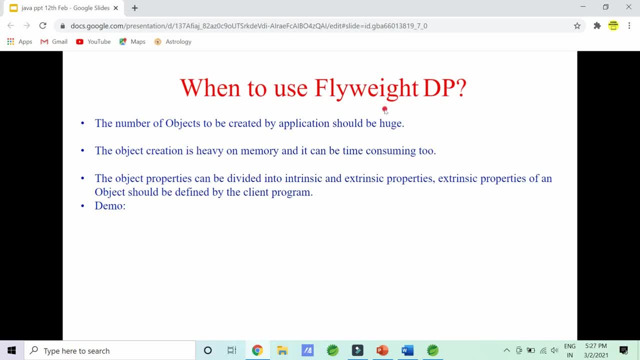 When This is a very important Interview question. please understand this carefully. When do you use the flyway design pattern in your programming style? So if you have a requirement which says the number of objects to be created are huge- suppose zoo management system- you have many number of animals- 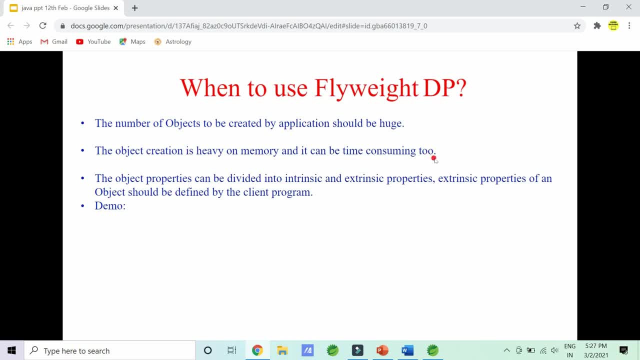 Now, object creations are heavy on memory and it is a time consuming too. The object properties can be divided into intrinsic and extrinsic properties. Extrinsic properties of an object should be defined by the client program. When all these three conditions fulfills, then you should go for flyway design. 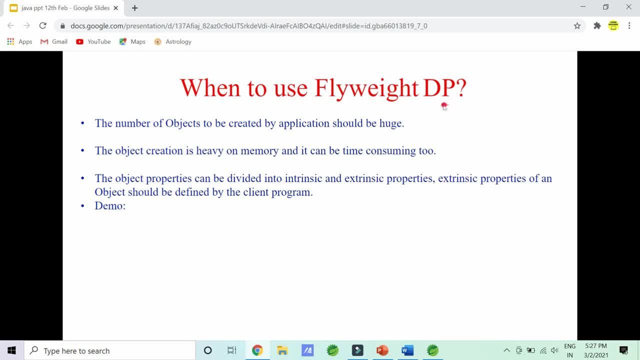 Pattern. What are these properties? What are these situations? The first large number of objects should be there. Object creation is a heavy memory issue and it is time consuming. Then go for design pattern And if you are able to divide your objects properties into many intrinsic 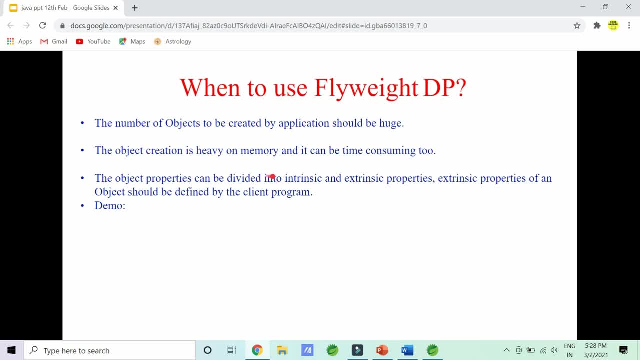 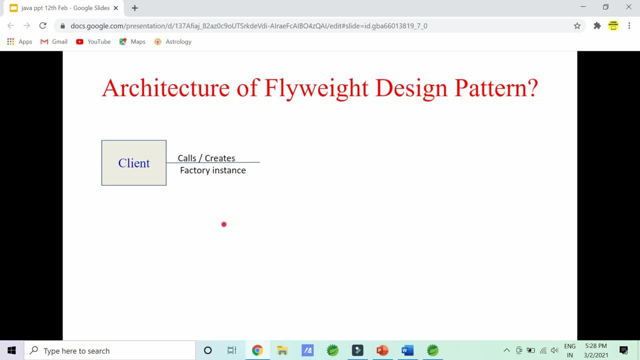 and few extrinsic properties, then go for flyway design pattern. If that is clear, let me quickly move ahead to the architecture of design pattern. OK, similar to that also you will have. you will be having a client which actually calls a factory. 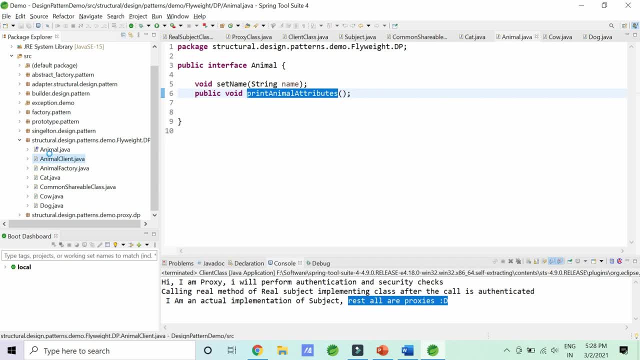 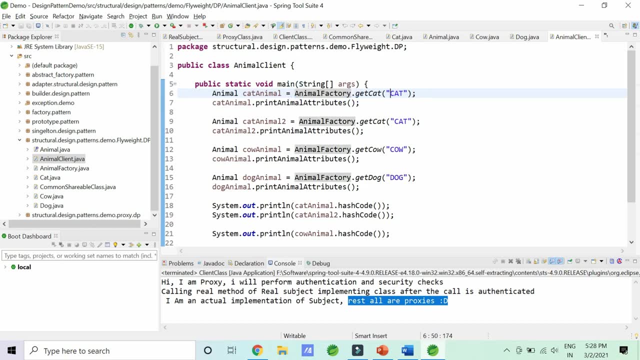 So let me tell you this is my animal interface. Now this is my client. Now client will have what Client will actually call the factory with a particular name. It's saying that I am a client, I want an animal object, Animal name of that animal is cat. 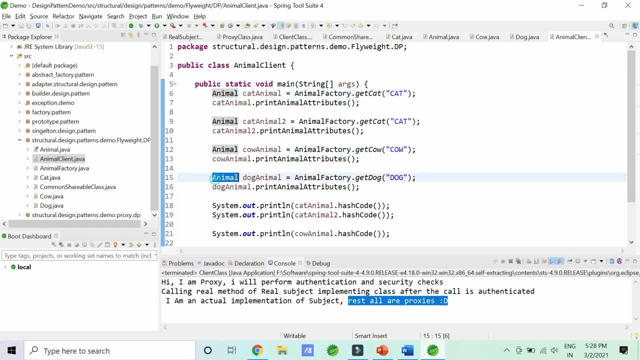 I am. I want an animal whose name is cow. I want an animal whose name is dog. Again, I want an animal who is a cat. So what? this is the client's requirement. So how it is implemented: keeping a one interface common. 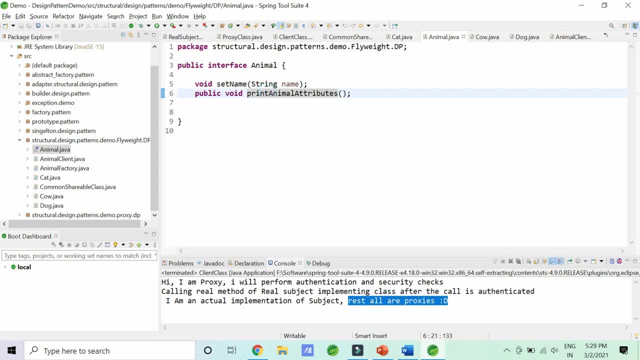 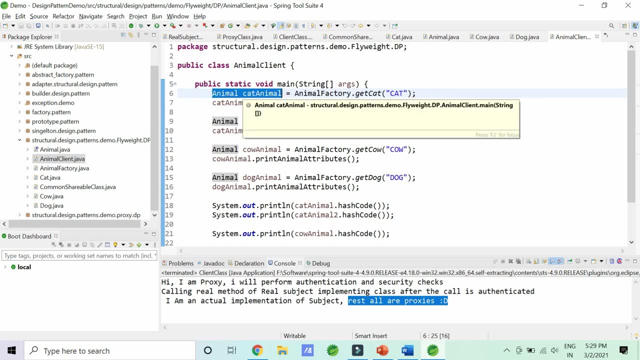 having the name and primary attributes which are the intrinsic or the common attributes. the client will say I'll create an instance or a reference variable of animal but factory will give me the real object. I'm not going to create any object with a new keyword. 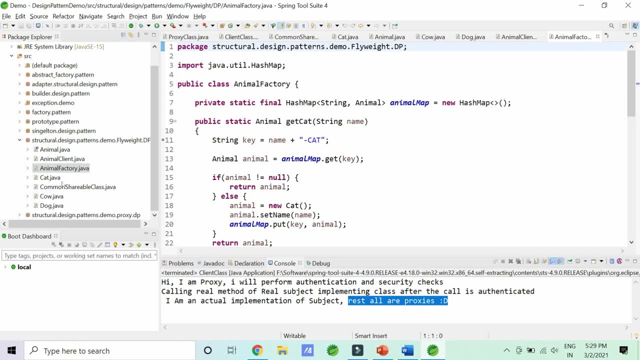 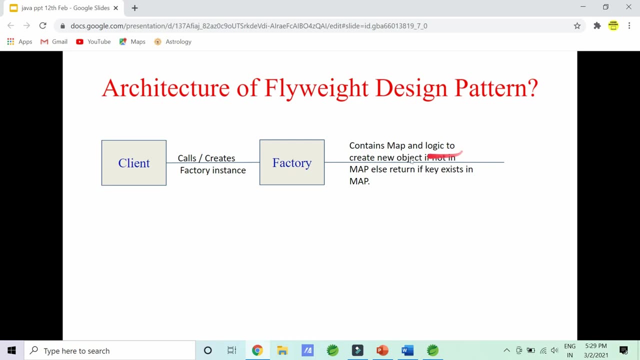 So what will factory do now, since it's a creating an object is a memory issue and a time consuming affair. So what I will do? I'll create a map here. So what factory will do? Factory will actually contain the map and logic to create new object. 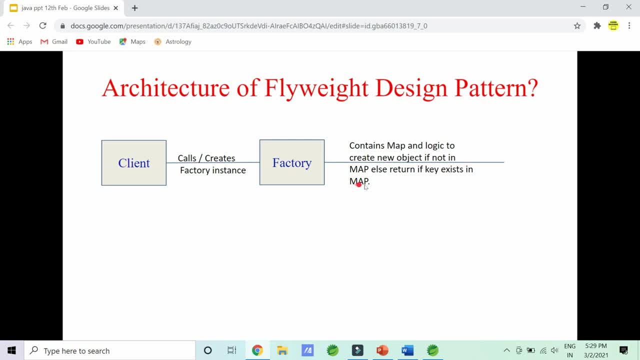 If not in the map, else return the key that exists in the map. It's difficult to understand. I completely understand. So I've given you an example. in the factory You will have one map. Can you see an animal map? So what will factory have a map. 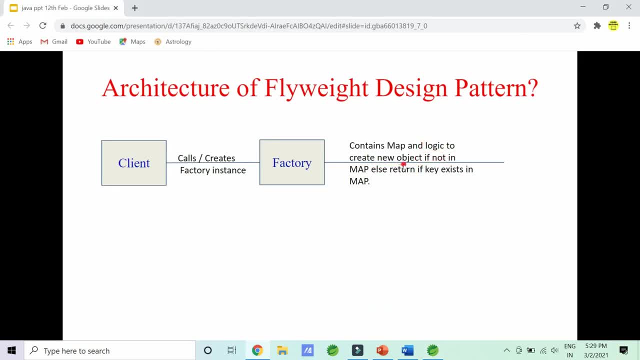 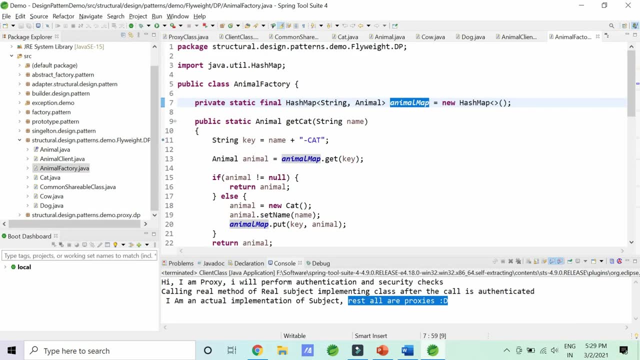 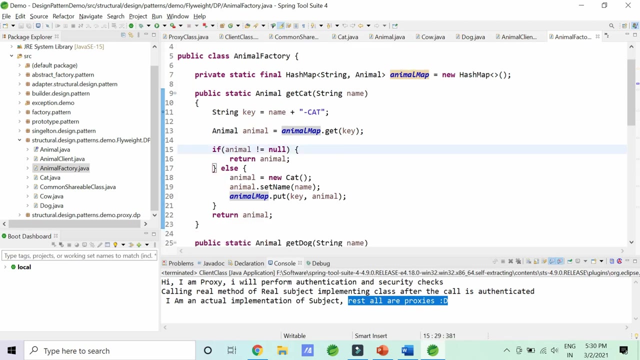 Then what will have it? a logic to create new object? only and only if new object is created if map doesn't contains it else, if it contains written that particular object. so it contains a logic to create a new object, but only and only when the given name appended with a key. 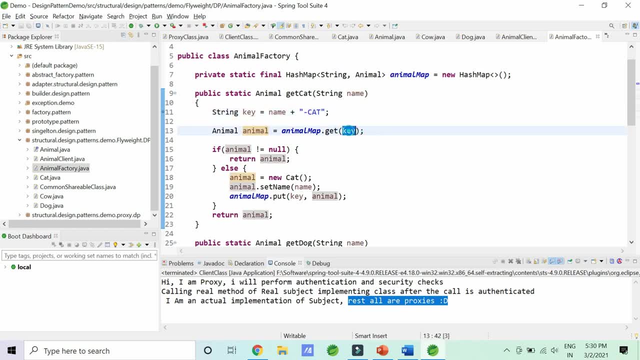 If key does, if that particular maps, if you try to get that key and it returns an animal. if it does not contain or it is not null, if the animal is already present, then return that animal, Do not create a new object. 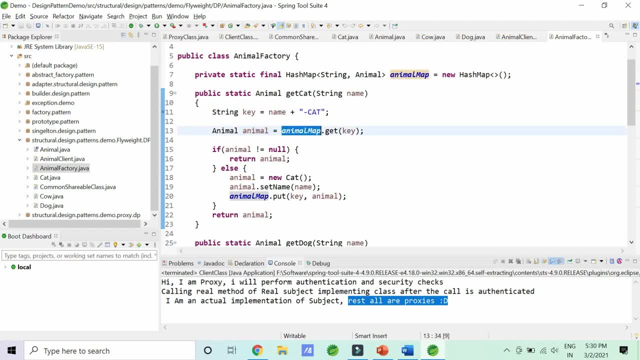 And if the map Doesn't contain any of the key, like cat and the score cat, then please create a new cat saying the name is cat and now put it in map so that again, if I try to get a cat, I should not create it with a new keyword, I should return it how it was. 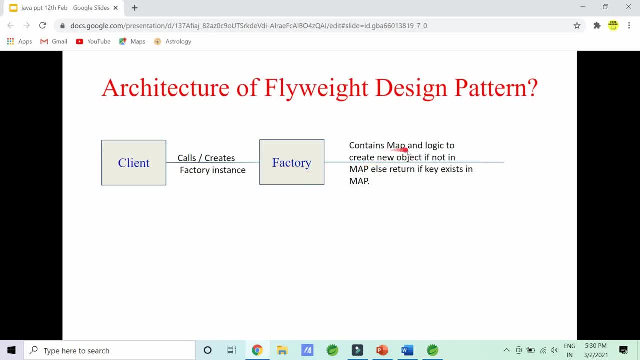 So what does factory contains? factory contains nothing but a map, animal map. It contains a logic to create a map, to create an object if it is not present in the map already. else, if it is not there, create a new. If it is there, please return the same. 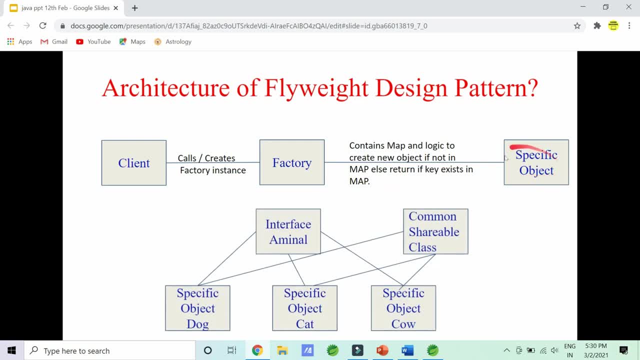 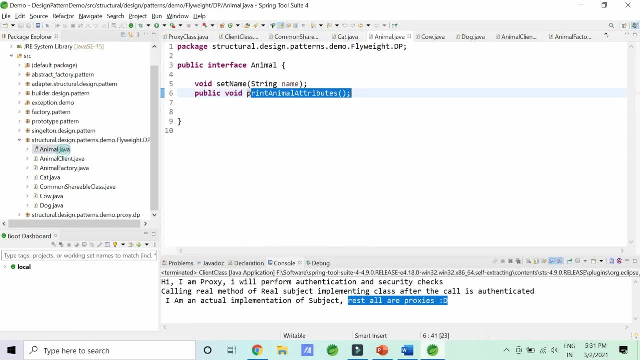 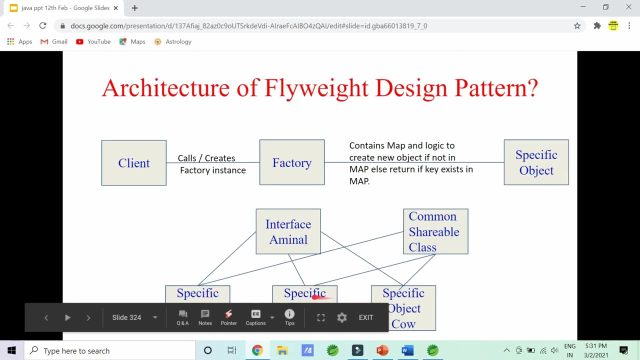 If that much is clear, You will get a specific object to the client. So, as per the discussion, your animal interface, this is an animal interface. It will have some properties, some some particular methods, which is implemented by specific cow, dog, cat, and they all have the common shareable also. 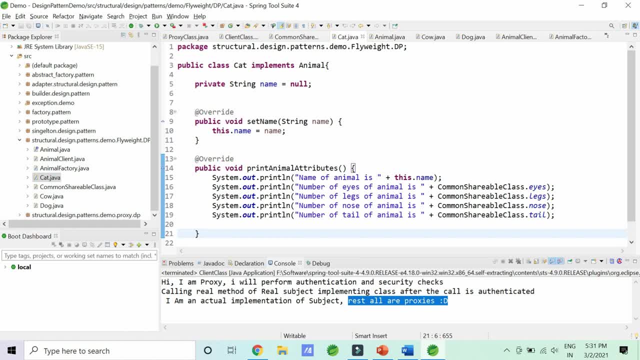 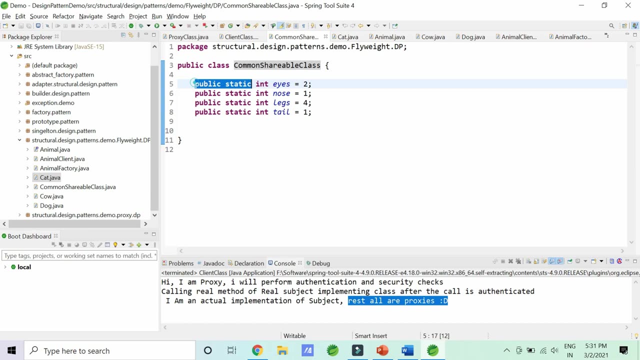 So cow, dog and cat does extend or does override. It implements the undefined method of animal. It says my name is this and will have an access to the common shareable for things in this class, that all these things are static, So you don't have to create an object or put a memory to the object. 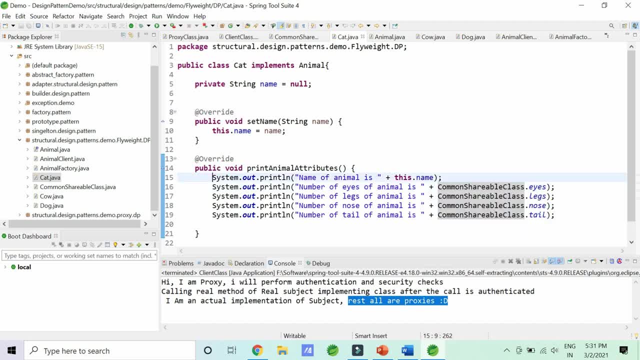 You can directly call it with the class name. So this is the way how you can actually showcase in an interview how to implement the design pattern. Now let me give you one example what I'm doing in client. So I'm trying to get a client. 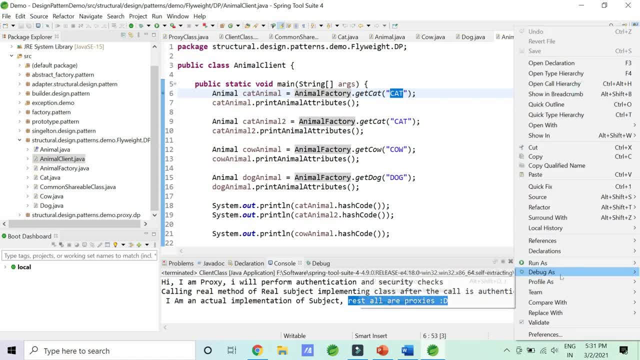 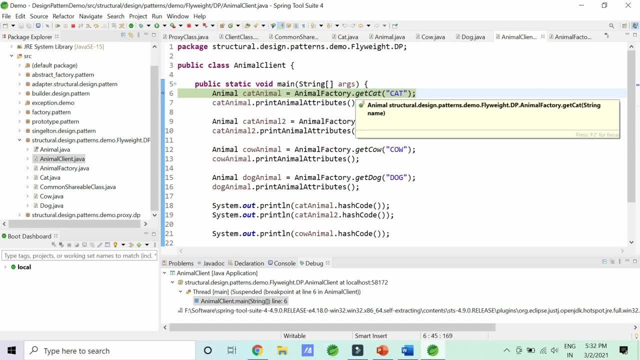 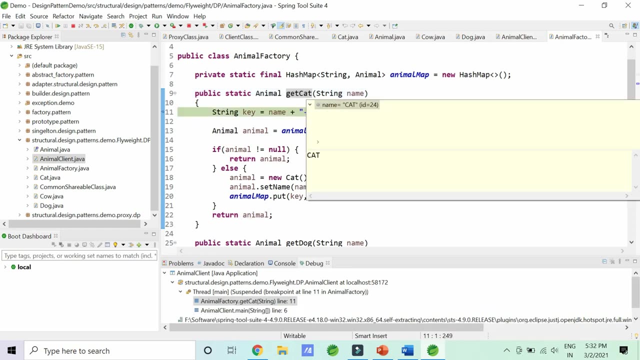 So let me actually debug this for you. It will be far easy for understanding. So here I'm creating a reference of cat animal and I'm saying: please go give me The cat object. So, as per the expectation, my cat came here. 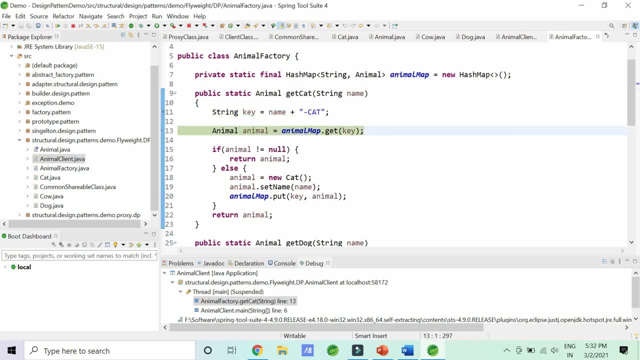 This is the name. Now my key will become CAT. underscore dash: CAT. This is my key Now. this particular map is completely empty right now, Right? So if I try to go and get the key, I'll get null. So, since it is null, it will create a new object. 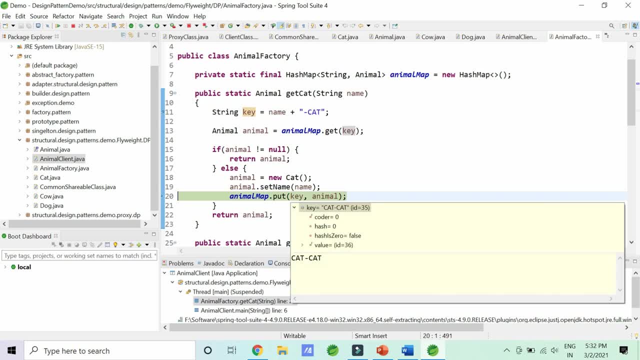 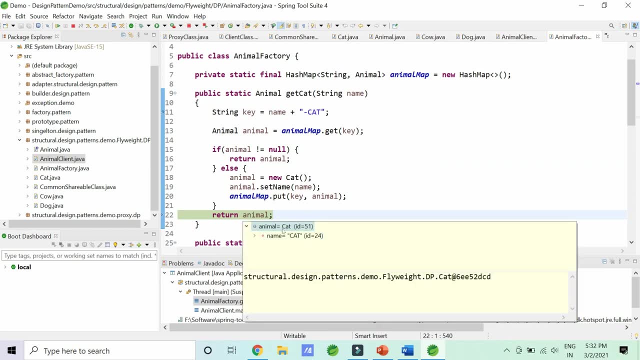 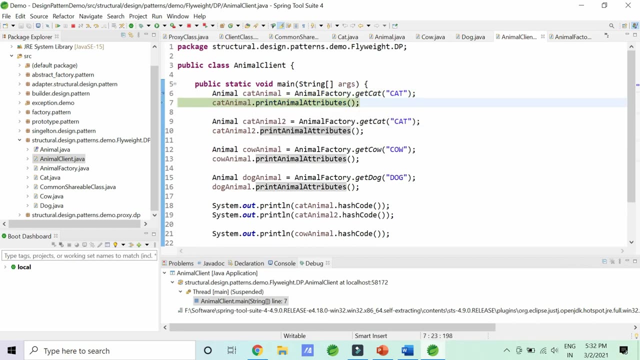 It will set the name as cat and it will put a key as cat, cat and animal as the particular object having a name cat, simple. And I'll have my object of animal, which is having a name cat. Now, if I try to go into this and print a particular 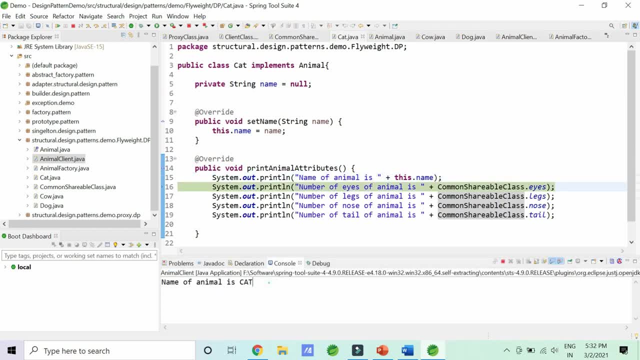 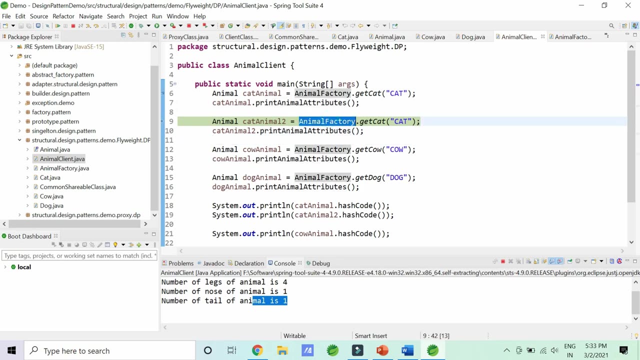 variable. so I'll get a name of the animal: is cat, The number of eyes is two, Number of legs is four, Number of nose is one and number of tail is one. This much is clear. Now what happens is I again go into the animal factory and say: give me a cat again. 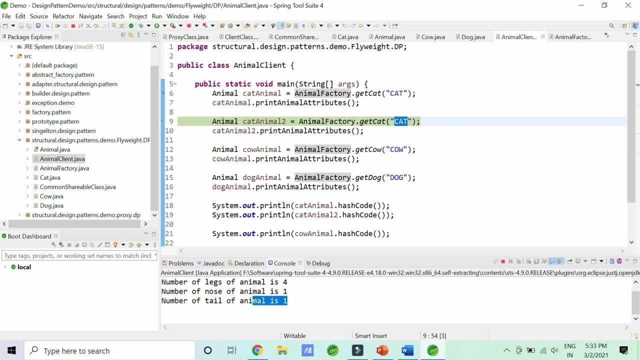 So what is your thinking? What will it to do? It will actually go and create object or it will return the existing object which is already created? that we will figure out when we will try to print the hash code. So if those two hash codes are same, that means we are not getting a different object. 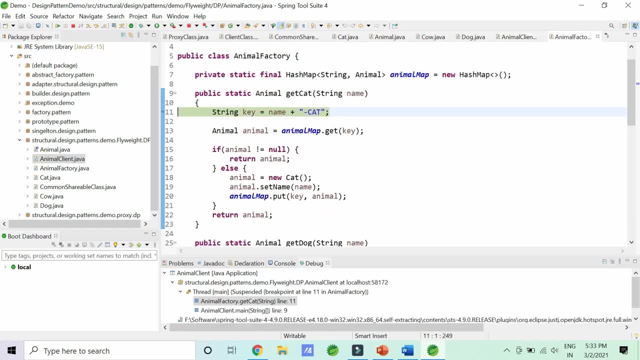 We'll get the same object. But since we have a debugger in hand, let me go into it. So my again. the name of the animal is cat. Now key becomes cat dash cat. Now if I try to get the cat dash cat, I got the animal cat because just two seconds. 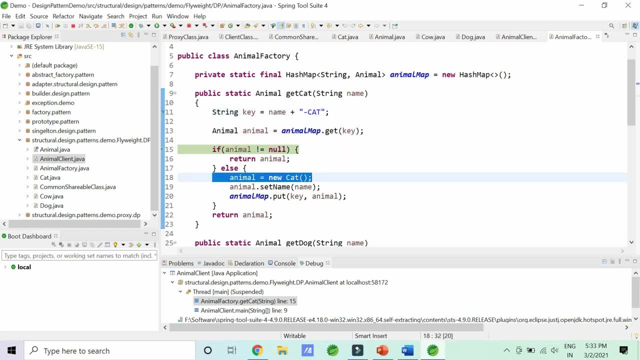 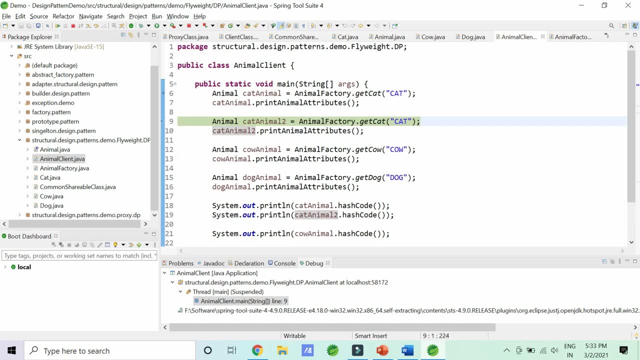 back. we have created object using new. now the animal map we have put there And hence we have. when I try to get it, I'll have my animal. Now the same object is written. Can you see no new object is created. We are returning from the same. 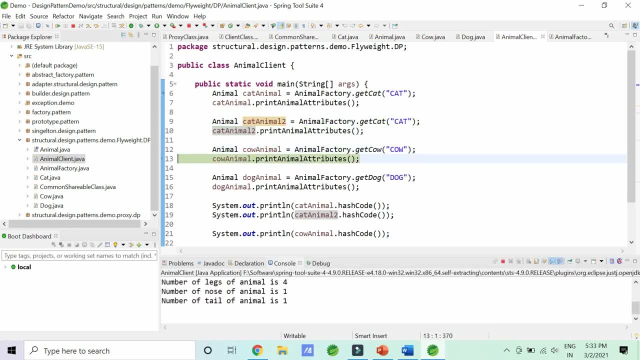 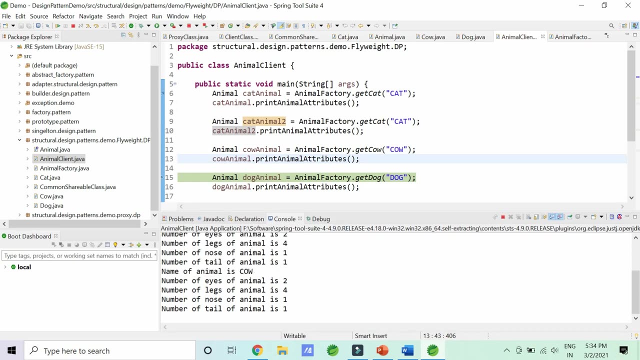 Now, if I try to print everything, the same thing will be printed The same, the name of the animal is cat and the same counting will happen. So I'm actually assuming that cow is again the same. So again, say is the name of the animal is cow. 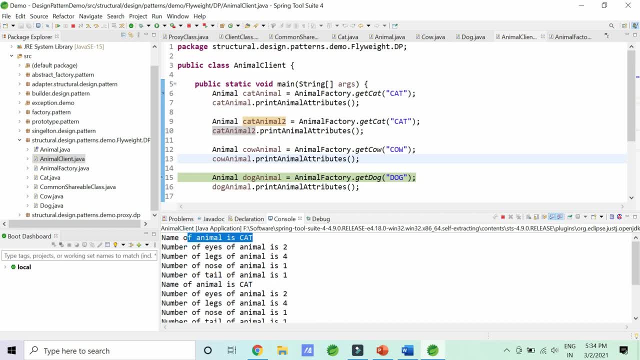 The name of the animal is cat. The name of the animal is cat. So can you see, if I try to call cat, cat and cow, this is what happens. The animal of the name is cat. The animal name is cat. The animal name is cat.